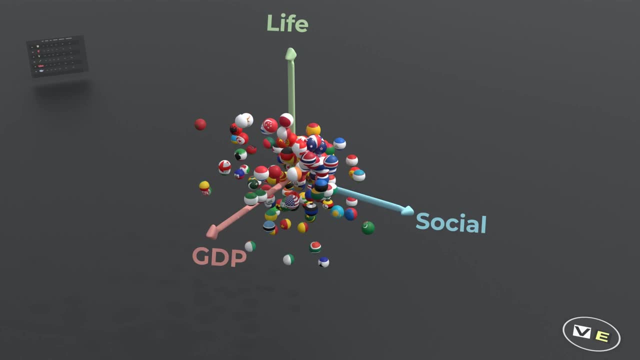 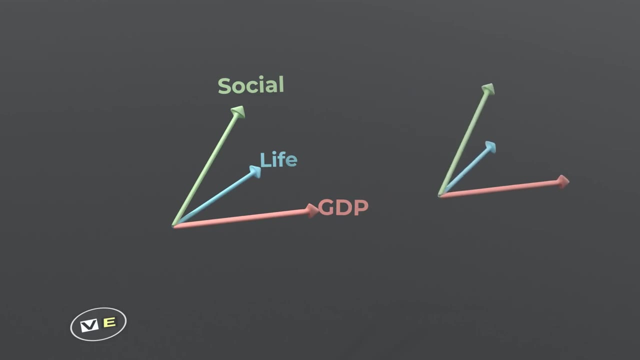 valuable information that might be contained in other factors of the data, like freedom or generosity. PCA is all about taking all factors, combining them in a smart way and producing new factors that are one and correlated with each other and two are ranked from most important to least important. These new factors produced by PCA are called principal components, and they are: 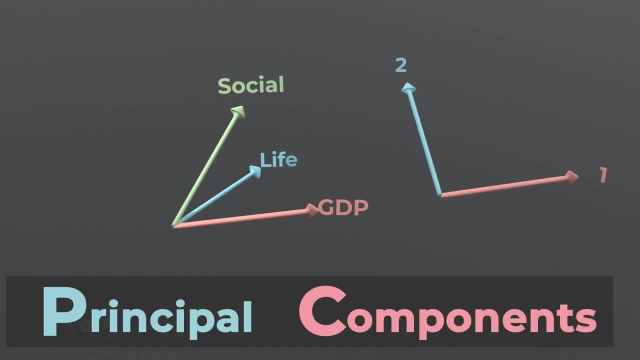 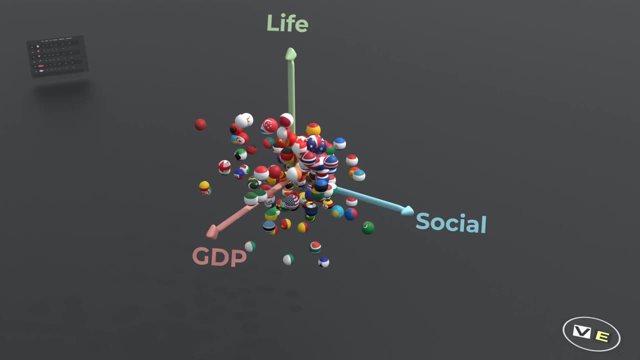 constructed in such a way that, if you restrict your attention to the first few components only, you would still get a faithful representation of the data. Let us now explain how PCA picks its components. For that, let's take the same data as before, but limit ourselves to the first three. 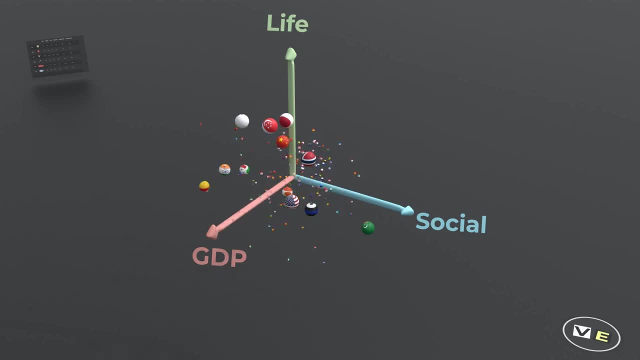 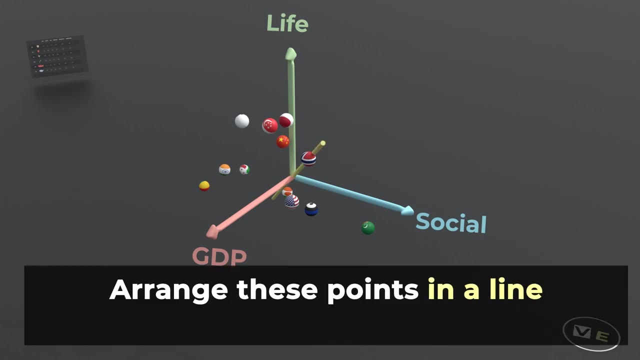 columns only for simplicity and drop a few countries so that the plot is not too cluttered. To pick the first component. PCA asks the following question: How can we arrange these points on a line in a way that preserves as much information as possible? A first attempt is to project all of 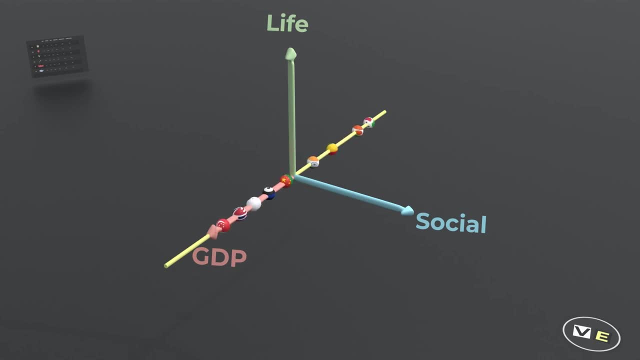 these points on one of the 3d axes, but that corresponds to throwing away a number of the other columns of the data. So maybe there is a better, less wasteful way To answer that question. let's take a small detour to explain how projection works When you project a point x on a unit vector. 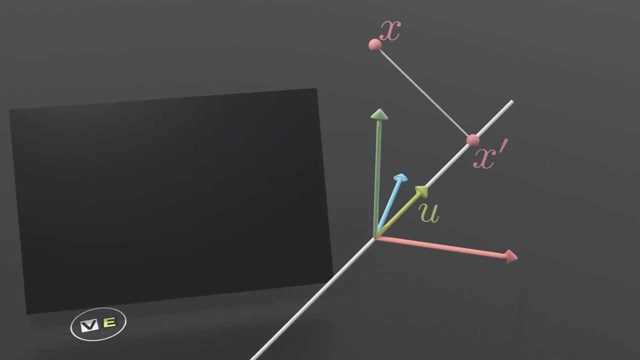 u, you get a new point, x prime, whose magnitude is given by the inner product between x and u, and we can think of the square of this inner product as the amount of information about x that is preserved after projection on u. In particular, this quantity is maximum when x is parallel to u and is minimal. 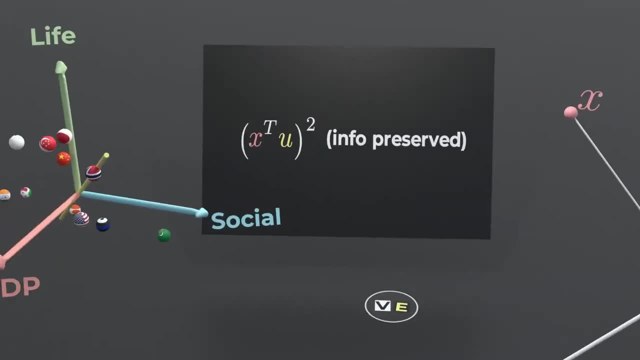 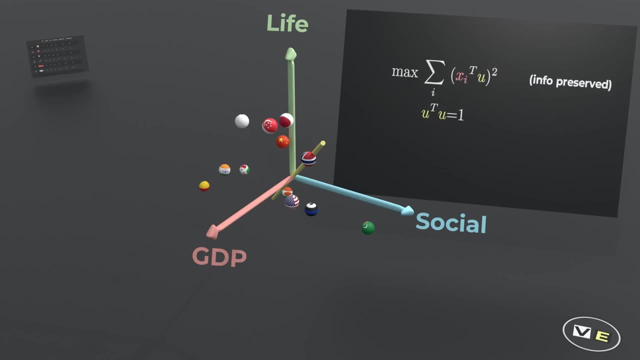 when x is orthogonal to u. To do this we need to take a small detour to explain how projection works. Back to PCA. the first component that PCA picks is a unit vector that tries to preserve as much information as possible, so it maximizes the sum over all countries of the square of the inner. 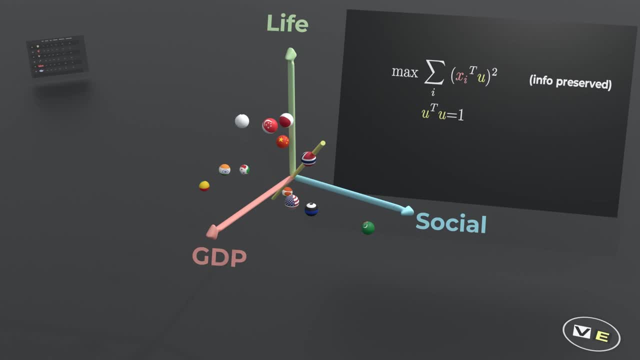 product. While solving this optimization problem might look intimidating at first glance, it is actually surprisingly easy to solve if you use the so-called Lagrange multipliers method. If you're not familiar with the terms optimization or Lagrange multipliers, you can either simply ignore the next 20 seconds and just take the results we're going to reach for granted. 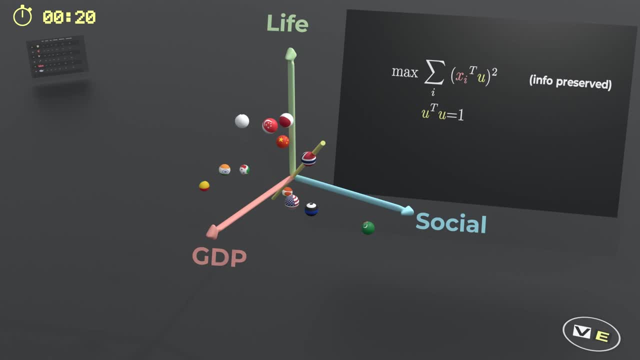 Or first go watch my beginner video series on optimization. So in order to solve this problem, let's simplify the objective function a bit. With some not terribly complicated manipulations, we can rewrite this expression as: u times the matrix, c times u, where c is known as the covariance matrix of the data. 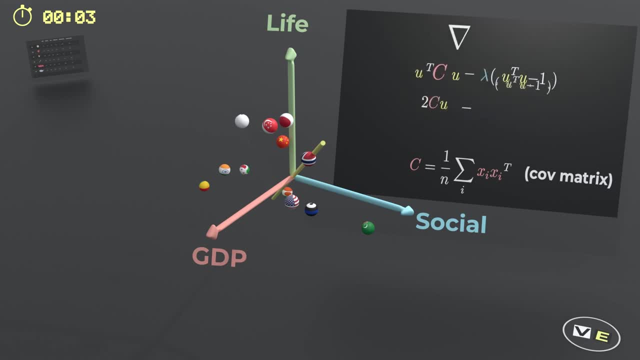 We then form the Lagrange function, take the gradient with respect to u and set it equal to 0.. In conclusion, we know that the direction u that preserves information the most after projection satisfies the equation. c times u equals lambda u for some unknown scalar lambda. 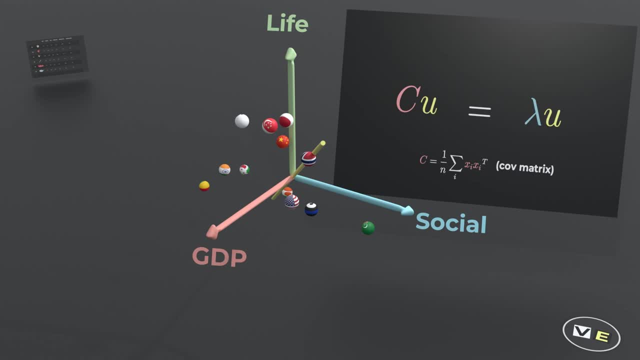 And if this equation looks familiar to you, there is a reason. This is exactly the equation of the eigenvectors and eigenvalues of c And, interestingly, the amount of information preserved after projection on an eigenvector is given by the corresponding eigenvalue. So clearly. 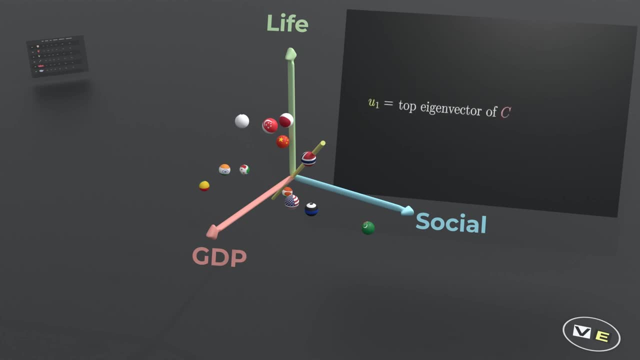 the best direction to pick is the eigenvector with the largest eigenvalue. So, for our example, this is what the eigenvector with the biggest eigenvalue looks like, And one way to interpret this component is that roughly all three original factors have equal contribution, and for this, 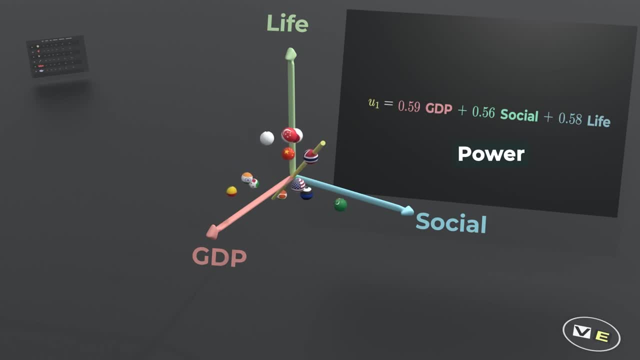 reason. let's call this component power. When we project the data points on this component, we note that Icelandic countries that we normally associate with happiness, like Norway, for example, are all positioned high on this axis, while countries like Niger are positioned low. Of course, this representation is not perfect, since you have countries like Singapore that rank high. 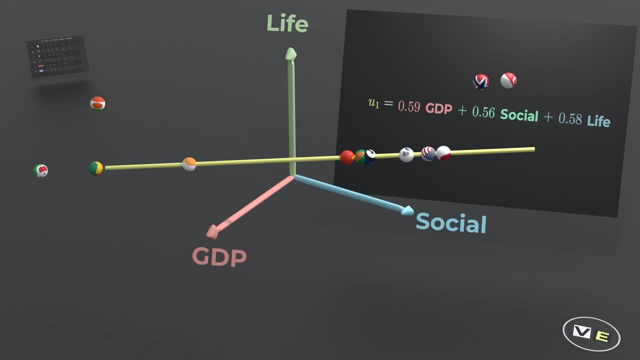 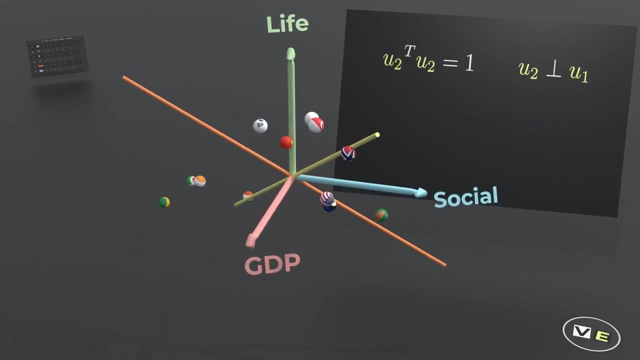 simply because they have an unusually high GDP. But this is to be expected, though, because we have only looked at the first component that PCA gives. Let us now discuss the other components of PCA. How do we pick the second component, for example? Ideally, the second component is a unit vector. 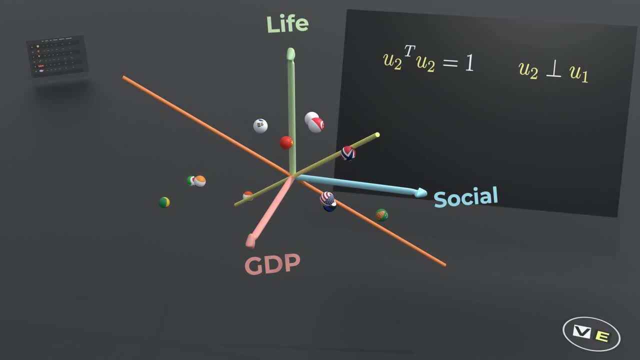 that does not contain information that is already contained in the first component. or, in geometric terms, we want the second component to belong to the subspace orthogonal to u1. So we can maximize the same quantity as before and, following reasoning similar to what we did before, we find that the second component is given by the second eigenvector of the covariance matrix.